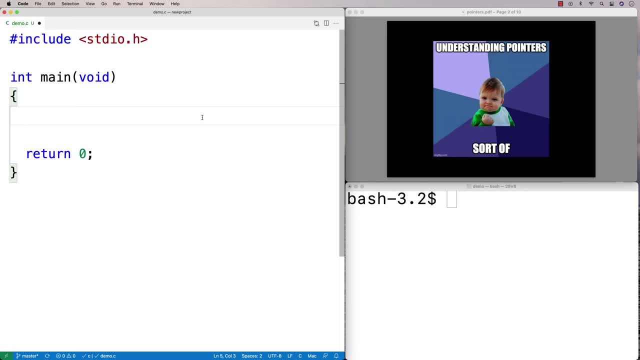 In this video I'm going to give an introduction to pointers in C. So normally with these tutorial videos I like to do live coding demonstrations, but pointers are tricky enough of a concept that it's going to benefit to do some visualizations. 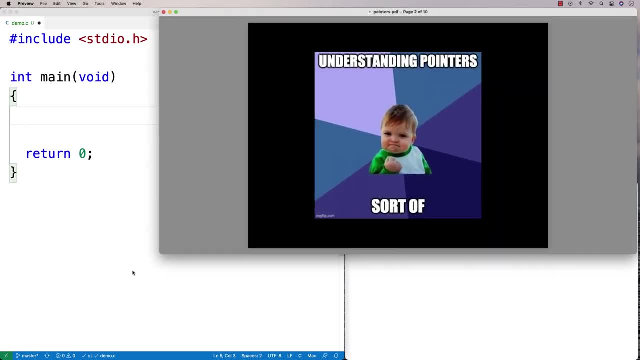 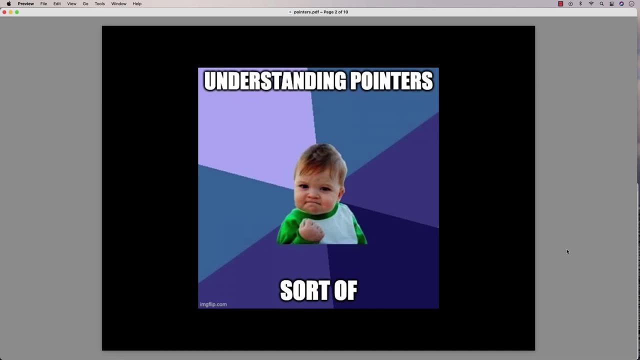 So I've made some of those as well. So, first off, when it comes to pointers, if you're having trouble understanding these, don't worry. Pointers are one of the trickier things to understand in C programming And, honestly, they're really one of the trickier. 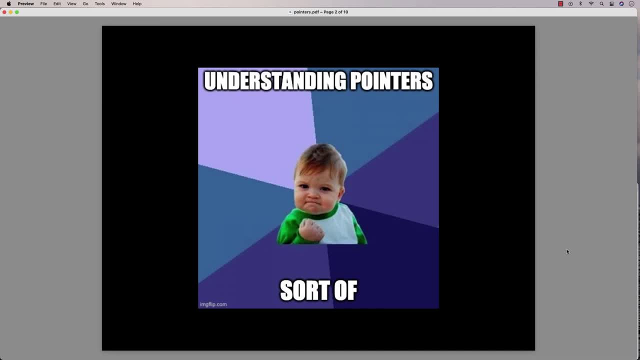 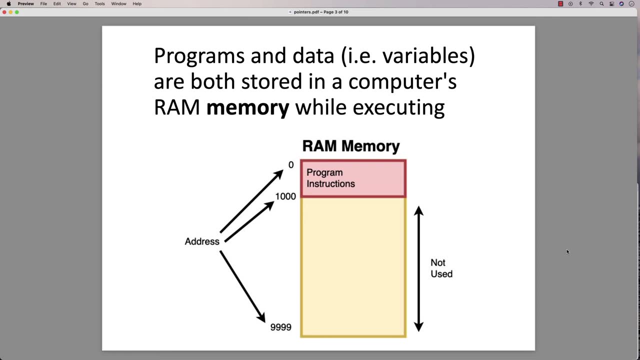 things you can understand in programming in general. They're just kind of hard to wrap our heads around. So what pointers are about is memory addresses, and normally our program and our data are stored in RAM And we can think of our program instructions as being stored in a. 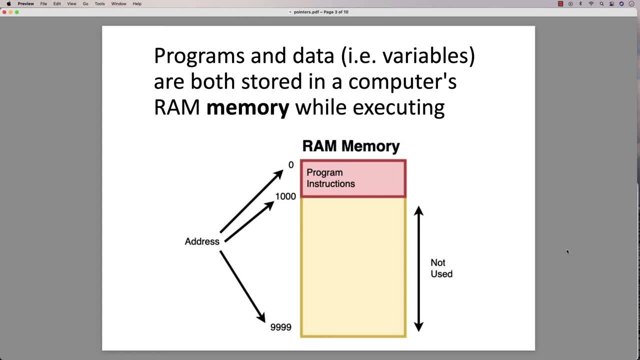 certain part in random access memory, the RAM you get on your computer. So when you get like a computer with eight gigabytes of RAM or 16 gigabytes RAM or whatever it is, that memory is RAM and our program is stored in that RAM. 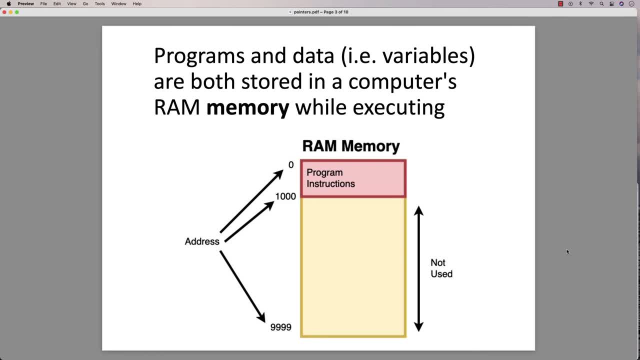 and data that our program uses like variables will also be stored in that RAM. And all the memory addresses, they all have some number, So like house numbers, right You have, like you know, 15 main street, 25 main street, a hundred main street. same idea with 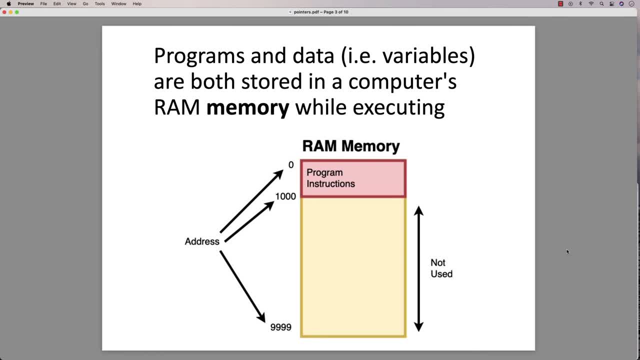 memory addresses. on a computer They have some number that is that specifies like that slot of memory, that position in memory, and memory just stores data. Memory just stores zeros and ones, essentially, And one of the things that stores is our program. But another thing it 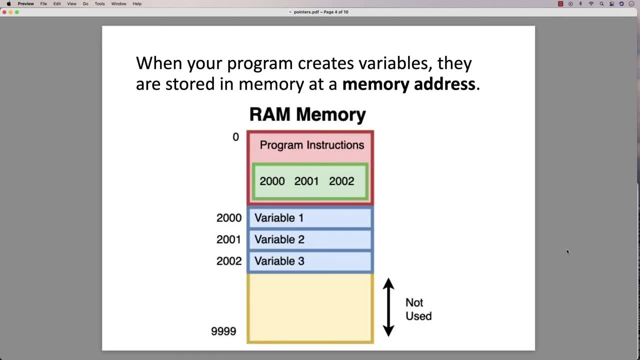 stores is our program's variables. So when our program creates variables, whatever they are- variable one, variable two, variable three- when our program creates these variables, those variables are also stored in memory. The data associated with them is also stored in memory. 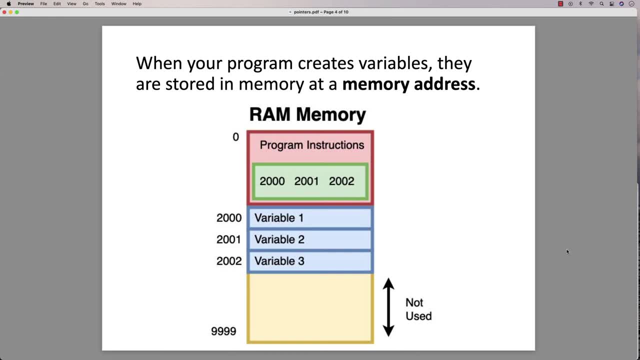 And so here we've got like variable one, variable two, variable three that have positions in memory, addresses of memory 2000,, 2001,, 2002.. And our program uses those addresses And really the variable is really kind of an identifier for that address. It's really a kind of like a name for 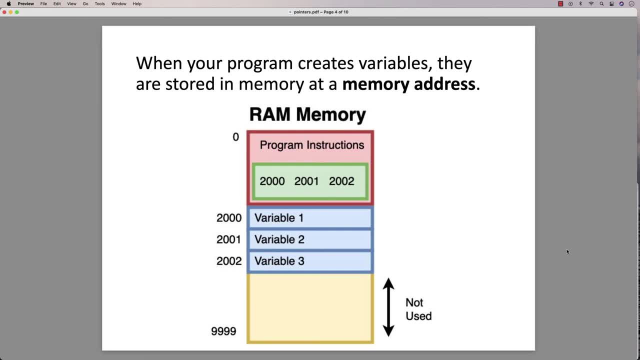 that address really. So you call it the variable one, variable two, variable three, And then you call it the variable variable X, but your program is really using memory address 2000 that the compiler has specified as being for variable X. Now, with memory addresses, they're gonna store some. 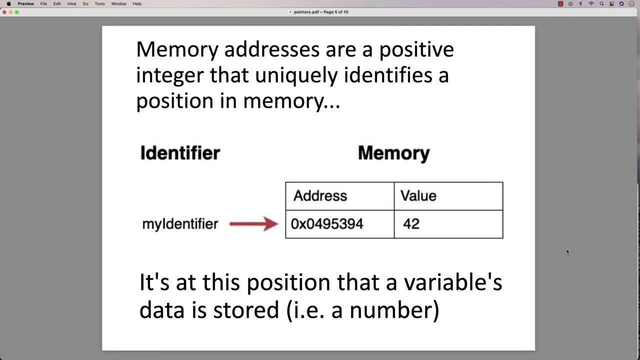 value. so, and it doesn't matter what really the value is- It could be part of a string, It could be an integer, it could be a double, but they're gonna store some value And we have some kind of unique positive integer for each of those variables And it's going to be a view value of 11, or 12, or 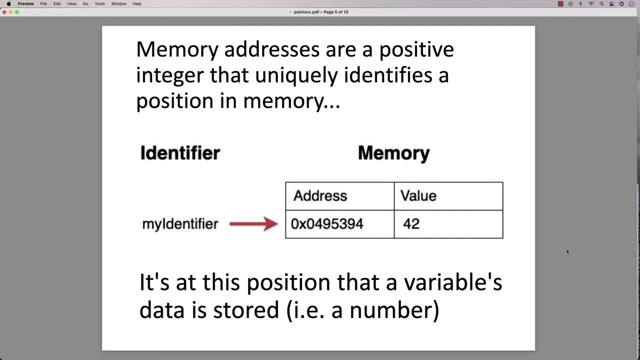 15. And it's going to be a key value of 11. And it's really going to give you a value of 11. And it's memory address. so when you have some variable like my identifier, that is actually really a reference for some address in memory and that's the. 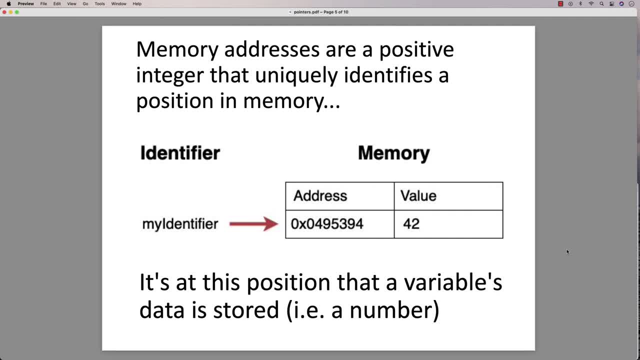 position where the variables data is stored, and it's gonna be. it's gonna be a number because, like all things, and computers are ultimately numbers, like zeros and ones. that number could represent a character or something like that, but it's ultimately some number there. now, when it comes to pointers, 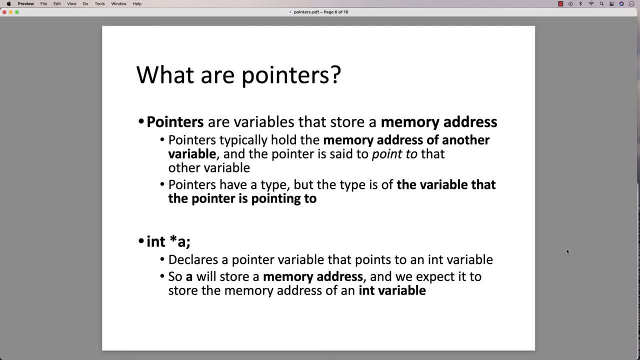 pointers are variables that store a memory address. so that's all. a pointer is. a pointer is a variable that stores a memory address. now, typically pointers are gonna hold the memory address of another variable and we're gonna say that the pointer points to that other variable. that's where the term pointer. 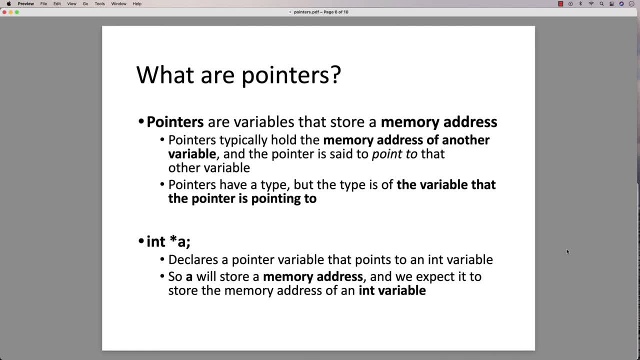 comes from and pointers have a type, but the type is actually of the variable that the pointer is pointing to. so the type of the thing that the pointer is pointing to. So if you have something like int star a, what that's going to do is it's going to declare a. 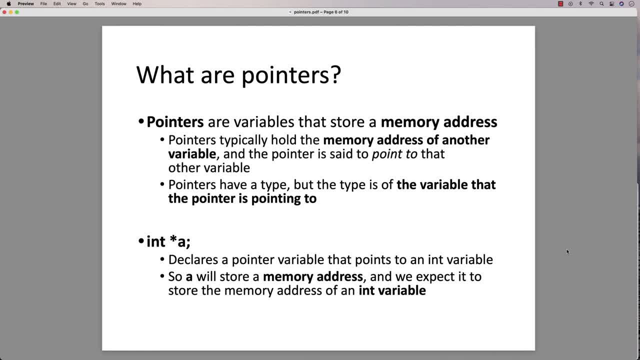 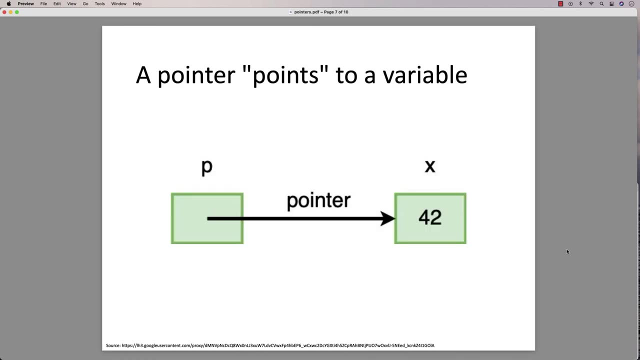 pointer, but it's going to declare a pointer variable that points to an int type variable in particular. So a will store a memory address and we expect it to store the memory address of an int variable. So we say that a pointer points to a variable when it stores its memory. 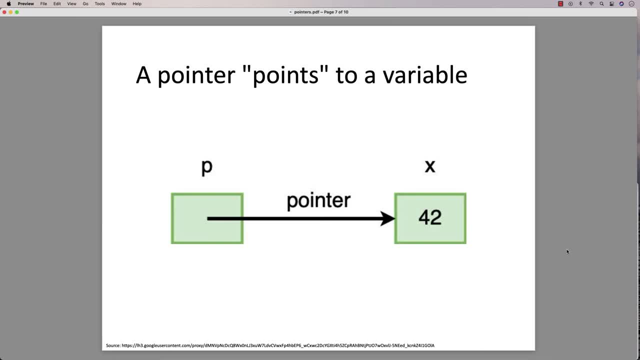 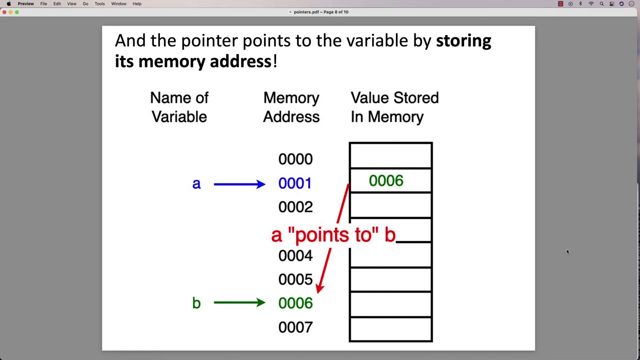 address. So if you have a variable x that stores the value 42 and p is a pointer and p points to x, then what p is going to store is the memory address of x. So it actually looks like this. So if you had, let's say, two variables, a and b, and they each have these memory addresses, like 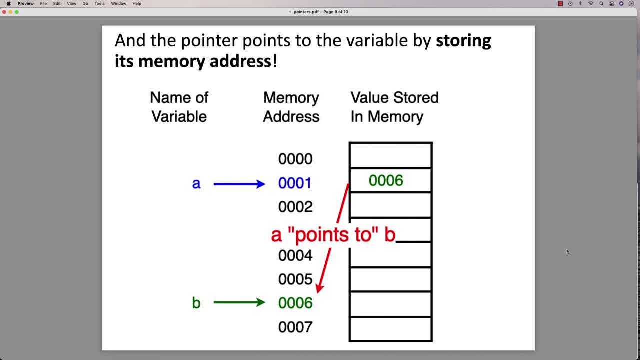 a has zero, zero, zero one and b has zero, zero, zero six. If a stores as a value at that memory address zero, zero, zero six, we would say that a points to b, because a is storing b's memory address, And so we would say a points to b. And that's what a pointer is. That's all really a pointer. 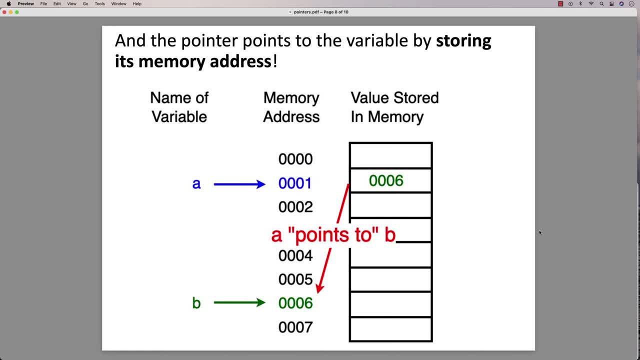 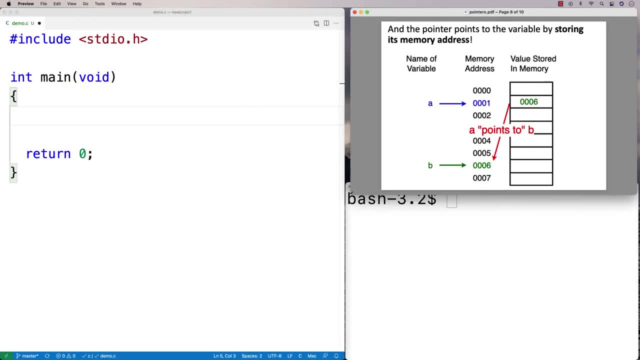 is is that a pointer stores a memory address, And that's the biggest thing you got to remember when you're trying to understand how pointers work. So let's actually code up an example of this now. So let's zoom this back and then we'll make some example pointers here. So let's make a 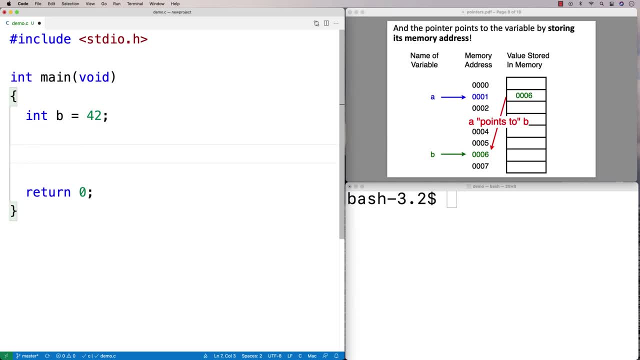 variable b and set it equal to 42. Then let's make a pointer a. So I'm going to say int, star a. So this is going to declare a variable a. that is going to be a pointer. So the star means that make a a pointer here And the int 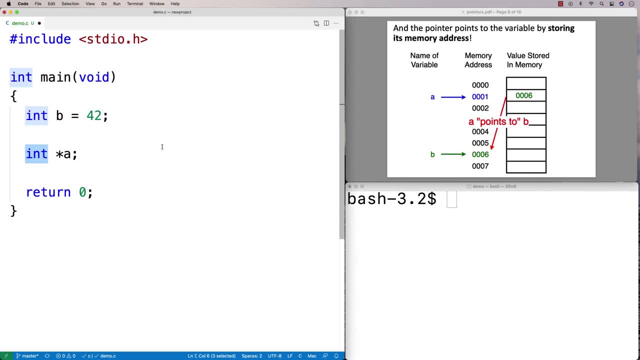 means that a is going to point to int values. Now, what we'll do to have a point to b is we're going to use this operator, and because to have a point to b, what we need to be able to do is have a store, the memory address of b. That's what we want to do Now, if we want to do that, 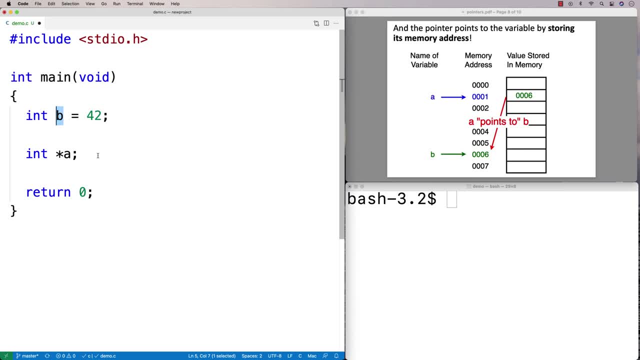 we want to have a store the memory address of b. We need some way of making a memory address of b And that's what this and operator does. So and and then some variable will give us the memory address of that variable. So I'm going to say: int star a is equal. 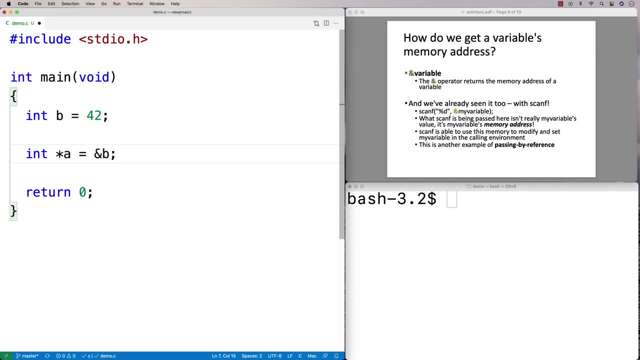 to and b. Now, at this point, a is pointing to b. So what does that mean? Let's print out the actual memory addresses to see what this means. If we do a printf. and I say, let's do a printf of a couple, 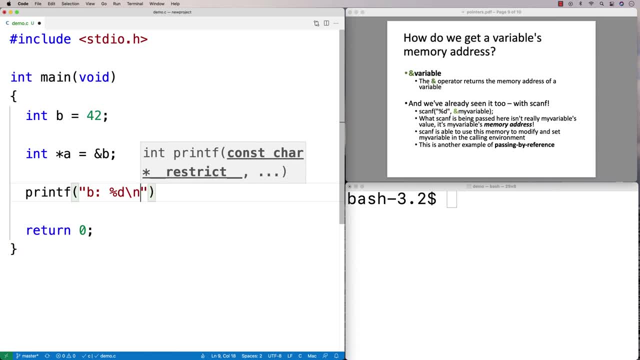 things. We'll say: let's do a printf of b. Just see what's inside b. b is going to be 42. We know that, But let's just print it out anyways. Then we'll do a printf of, we'll do and b And we'll do. 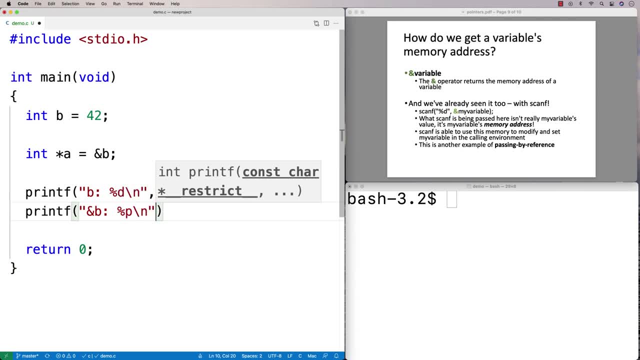 percent. I'm going to say percent p here. Percent p is how you can print out a pointer, value or a memory address, And I'm going to say and b, Then I'm going to do printf And I'm going to do printf. 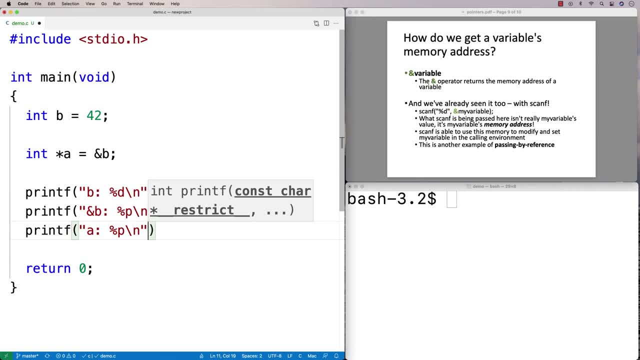 of a And I'm going to say percent p slash n, And I'm going to say a, And so we're going to print b and the value of a, And the value of a is going to be the memory address for b, because that's what 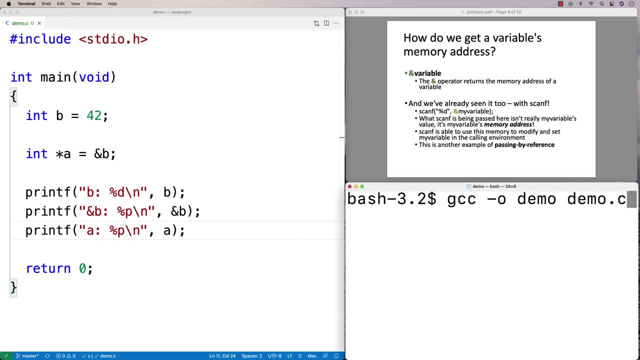 we set it to. So let's do a compilation here and then we'll run it And we get that b is 42 and b is this value, And you can see that a stores that value. They're the same. Now what this means. 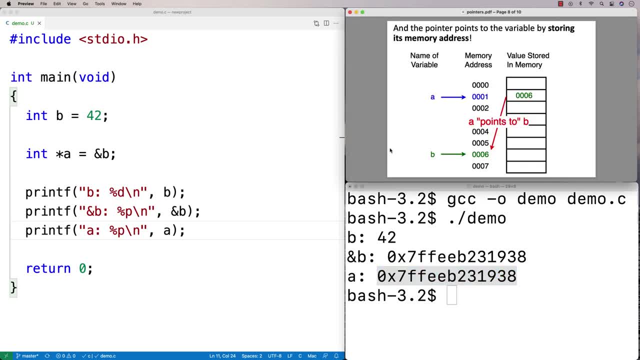 is that we have this situation now where a is storing the memory address of b. Now, when we've got that, what that means is that we can actually use a to modify the values, the value of b, So we can actually use the pointer to actually access the value contained in b. So to do that, what we're 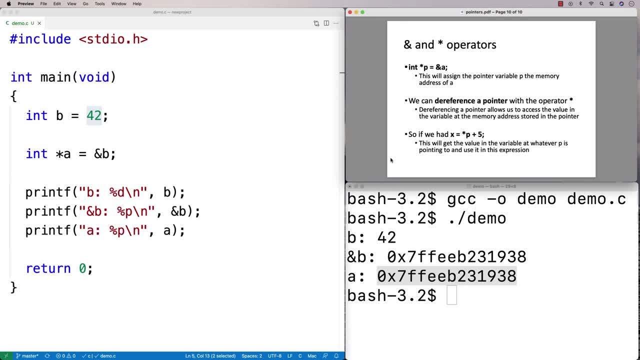 going to use is the star operator. So the star operator allows us to what's called dereference a pointer. When you dereference a pointer, you're accessing the value in the variable at the value of a. So we're going to use a pointer to access the value contained in b. 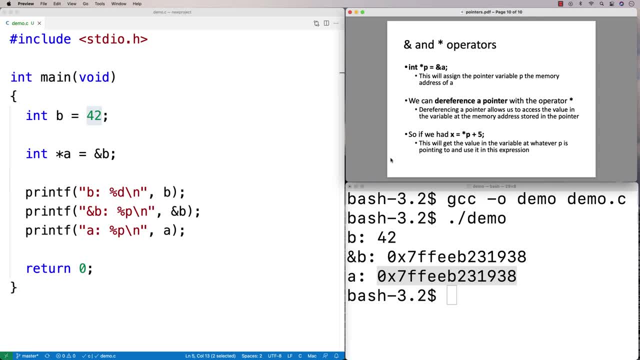 You're accessing the memory address stored in the pointer. You're accessing the data that is being pointed to. So we're going to say this, We're going to say here: star a is equal to, And I'm going to say here, 50.. Now let's print out these things again. Now let's print out b and these. 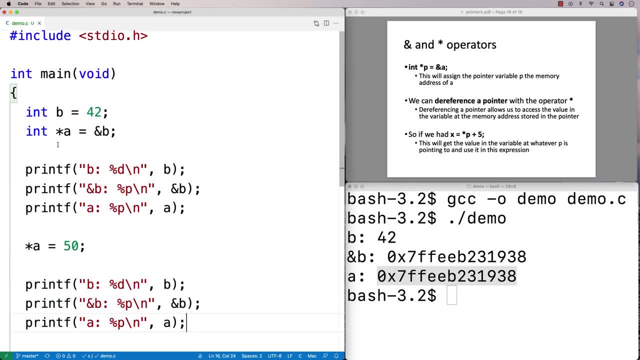 different values here again. So we'll print them out again here And we'll do a clear. And I'm just going to go in here now And I get here: b is 42 and b is this and a is that. But now I've changed. 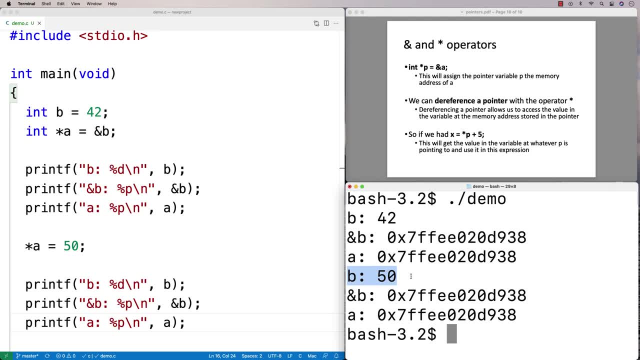 b to 50. How did that happen? I never said b equal to 50. And yet now b is 50. And b is still the same before, And so is a, even though I said that a is equal to 50. So I didn't say a is equal to. 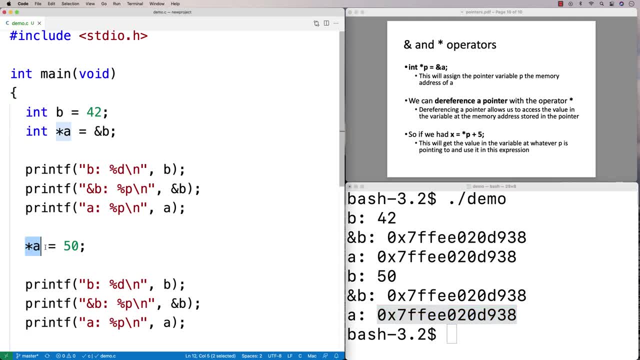 50. I said star a is equal to 50. And star a basically says: go get what a is pointing to and use that. And we can use it in expressions or we can use it in assignment statements like this, where I'm saying like: go get what a is pointing to and modify that. So it's kind of like if we 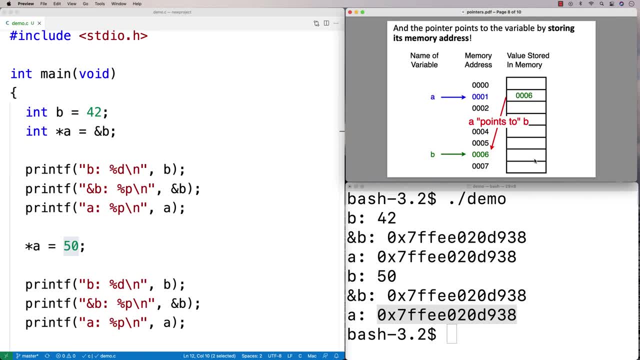 had you know on this in this graph. here you know, when I say star a, I'm saying don't modify a, I'm saying modify b, Modify what a is pointing to. And that's what dereferencing a pointer does. 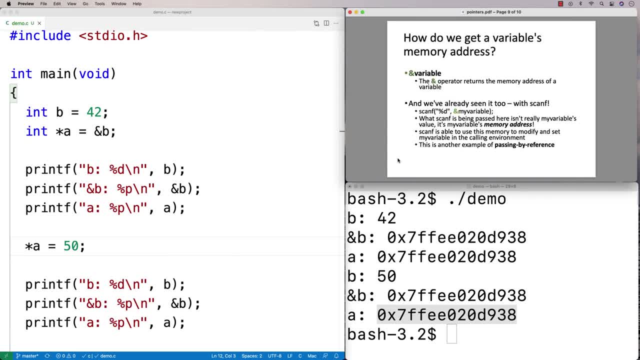 Dereferencing a pointer goes and gets what the pointer is pointing to and works with that. Those are the two operators that really matter the most for pointers is the and operator and the star operator. And again the and operator gives you the memory address of a variable, The star. 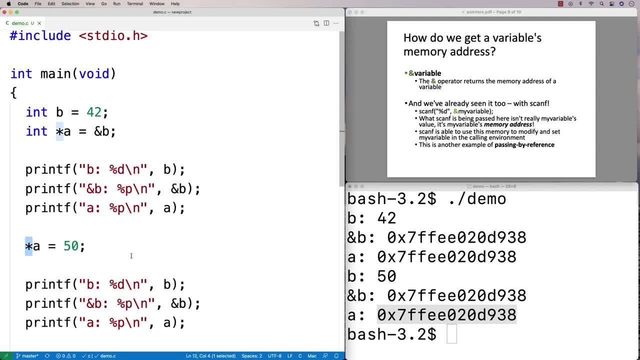 operator is going to dereference a pointer and go get what a pointer is pointing to, And we'll let you work with that. So why do this, though, Like, why have a variable that is a pointer to another variable? What's the purpose of this? So there's two big reasons why we use pointers in C. One is: 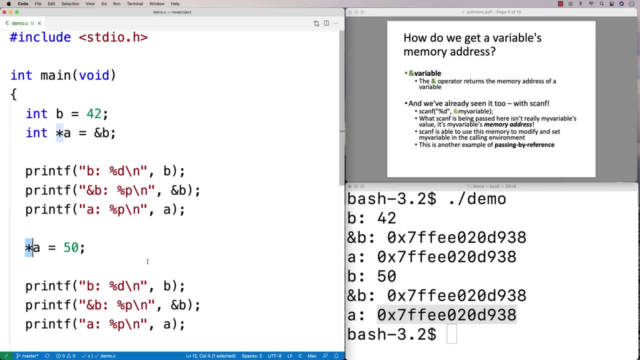 to do what's called pass by reference or, more accurately, pass by pointer. And that's when we use pointers to allow us to make a function that can actually modify multiple variables at once. And we actually have an example of this already, if you think about how scanf works, And I'll show. 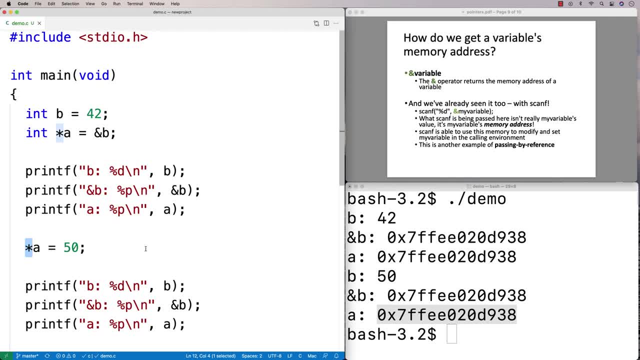 you an example of that. Now, another reason why we use that is what's called dynamic memory allocation, And that's where we can allocate space for things we want to use in C with a varying amount of space at runtime. In other words, we can decide how much space to allocate something for. 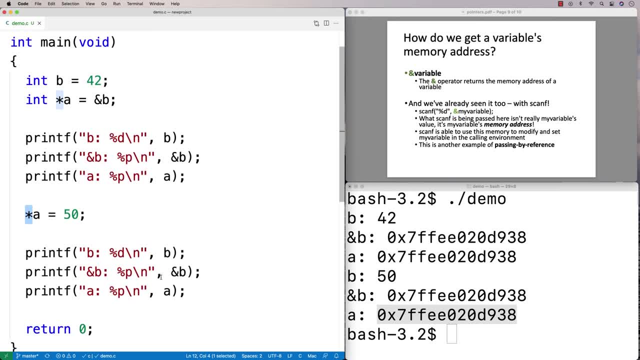 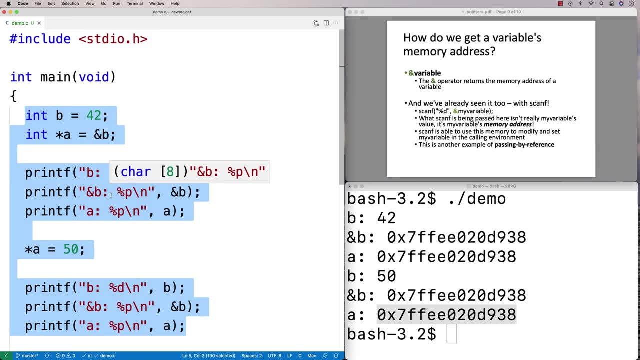 something as our program is running, And I'm actually going to make tutorial videos for both of these concepts separately, because they're both big enough of a concept that we should cover them separately, But I'm going to go over the ideas somewhat in this video as well, Just that way. 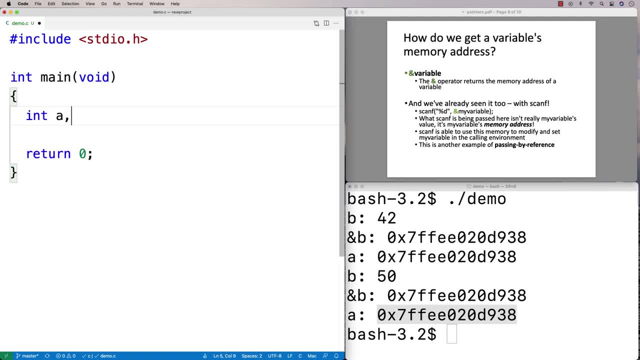 you can see why we're going to actually use pointers. So I'm going to say here int a, b, c, and I'll say a is equal to b, is equal to c, is equal to zero, just to initialize all of them to zero. I'm not sure if you know you can do this or not. in C, 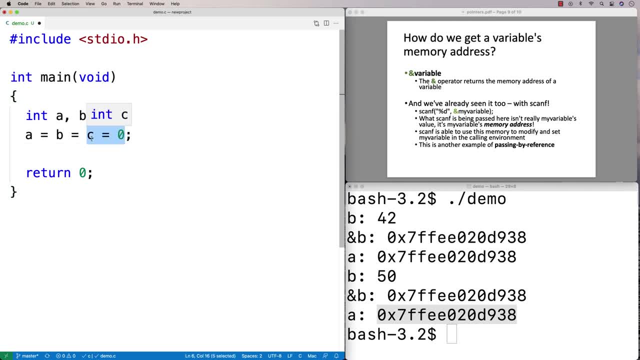 but if you set c equal to zero, the result of this is going to be zero. It's going to return zero essentially, And then b is going to be set to zero, And then a is going to be set to zero. So this actually sets all of them to zero, just to initialize them. So let's do an example though. 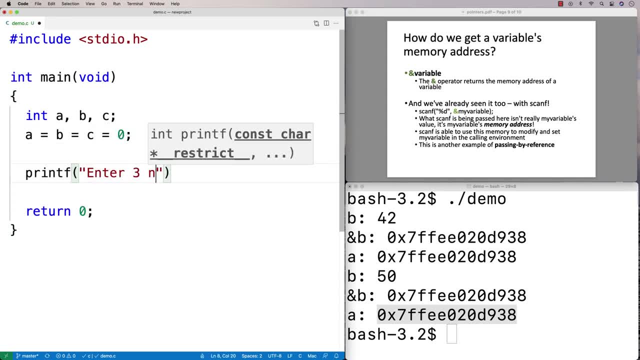 I'm going to say printf and I'm going to say enter three numbers, And we're going to ask the user to enter three numbers. Then I'm going to use scanf here And I'm going to say %d, %d, %d, And I'm 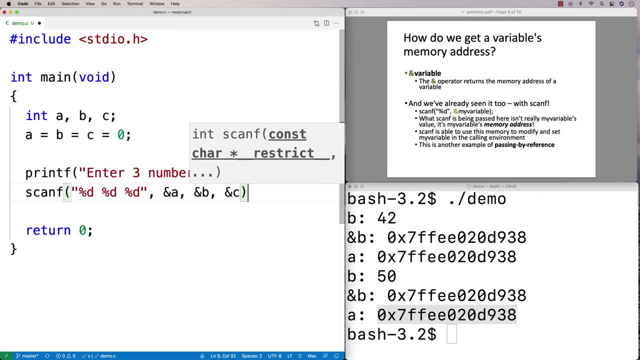 going to say here and a and b and c, And then I'm going to say printf and I'll say result %d And I'm going to add together a, b and c and print out that as a result. So what's going on here with scanf is that I'm giving it here and a and b and a and c as 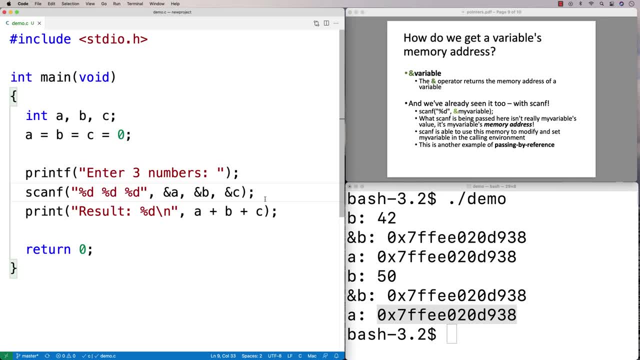 arguments. Now, if you've never seen scanf before, what it allows us to do is receive input from the user and, amongst other things, It can also receive input from standard input. it's called So it can actually do a little bit more than that, But what it's doing in this case here is it's going to 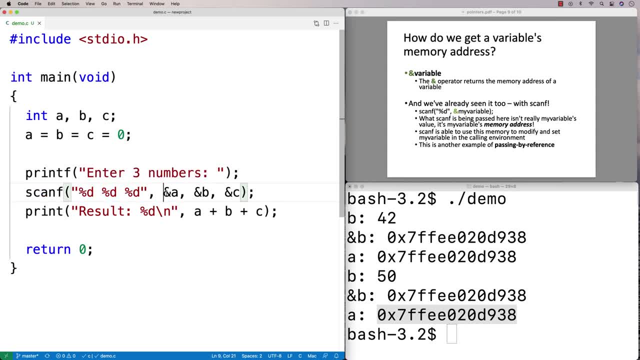 accept three numbers from the user, And it's going to accept three numbers from the user, Three integers, And we're going to store them into a, b and c. So how is this that the scanf is able to modify a, b and c? How can it do that? And we'll give it a test here, just to see that I'm 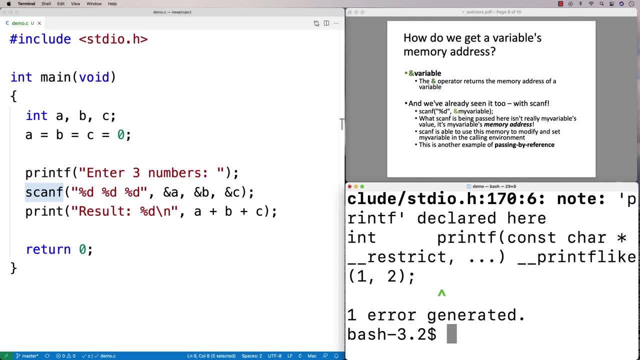 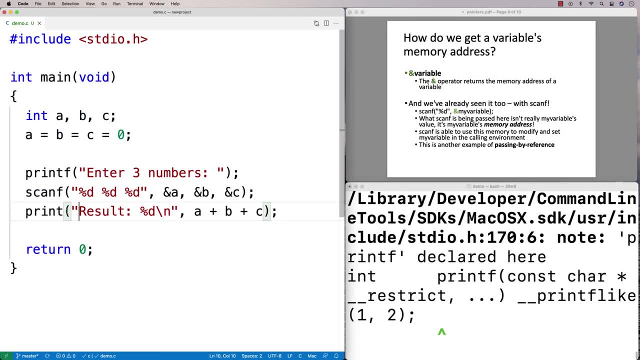 not making this up here, But scanf is going to be able to modify all these variables here. And if I, oops, did I mess something up here, What did I do here? It says: oh, I forgot to say printf here. 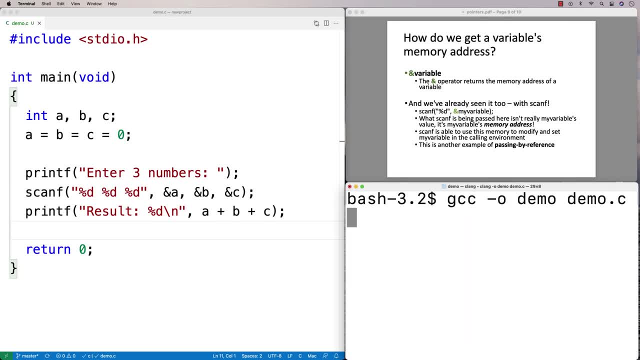 I just said print. I'm thinking of Python or something here. So, okay, we'll compile it again, because I'll say 5,, 10,, 2. And we get 17 as a result here, And what's going on here is scanf is. 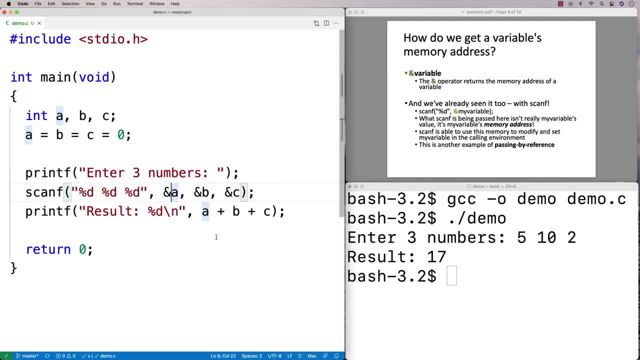 modifying a, b and c. The reason why it's able to do that is that we're not passing a, b and c to scanf. When we pass arguments to a function, what the function gets is the value of that variable or that expression or whatever we've put as an argument. So if I were to say like a here: 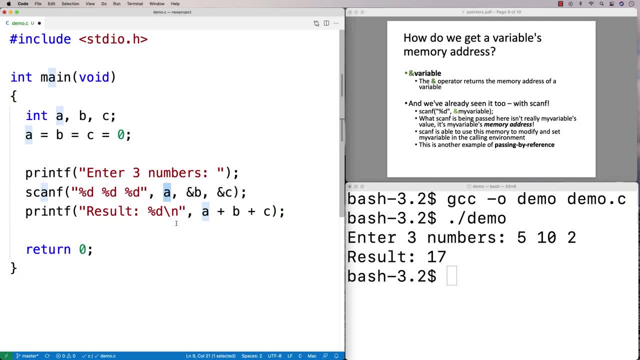 pass in a, what would be passed in is zero. That's the value of a. If I say and a, what gets passed into scanf is the memory address of a, And scanf is able to use that memory address to modify a, And this is what's called pass by. 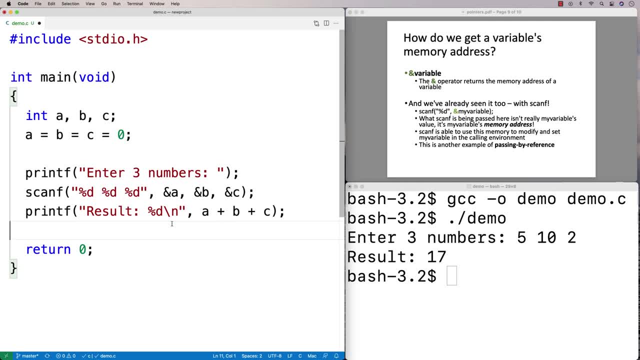 reference Or, if we really want to get technical, it's called pass by pointer in c, because we're using pointers. Pass by reference is technically slightly different, but most people just call it pass by reference in c. anyways, Let's make our own pass by reference function in c using pointers. 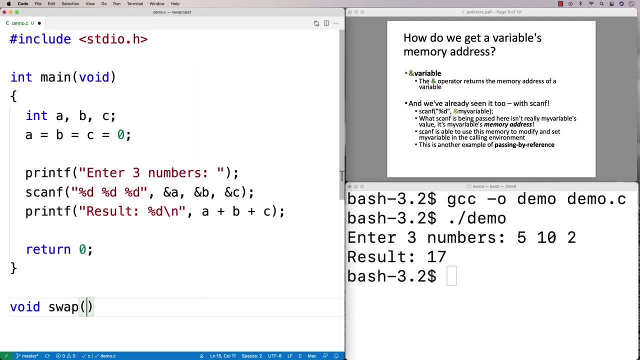 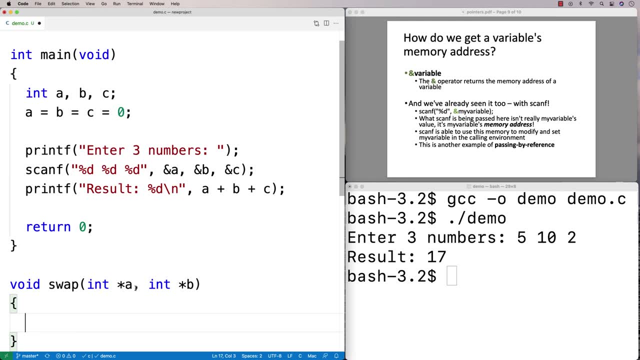 So I'm going to make a function, I'm going to say void swap, I'm going to say int star a, int star b. So it's going to take in two values and we're going to swap these values. But what it's going to take in is actually memory. 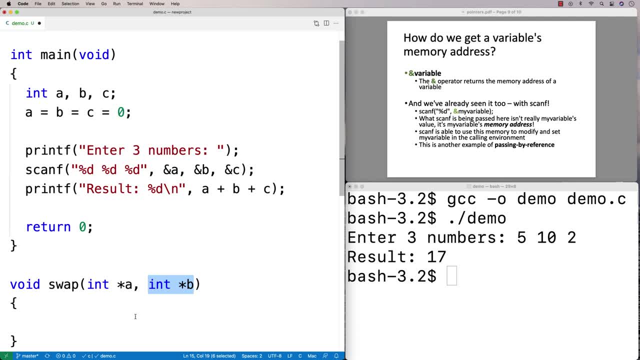 addresses. So it's going to take in memory addresses that point to those values we want to swap, And so the value in this case is actually going to be a memory address similar to scanf, And we're going to use that pointer to actually swap the variables. So I'm going to say here: int. 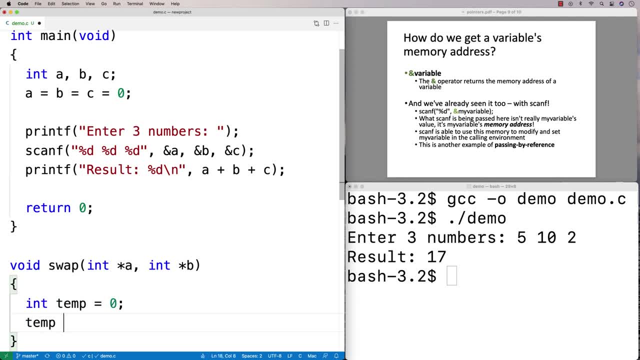 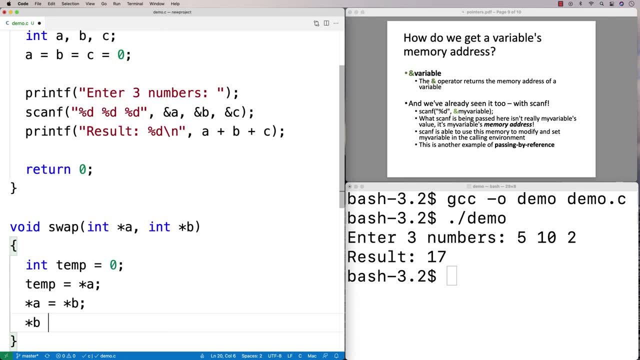 temp is equal to zero, I'm going to say temp is equal to star a. i'm going to say star a is equal to star b. then i'm going to say star b is equal to temp, and we're going to use this function here to swap two variables using 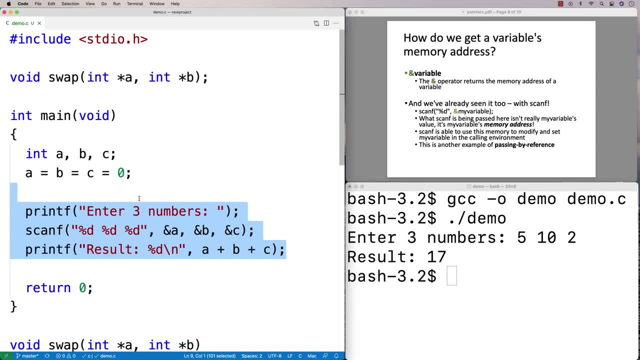 pointers. so let's actually make a little test of this now. i'm going to say here int a, b, or maybe i'll make them different, just that way it's clear. i'll say int x, y. i'll say x is equal to 5, y is 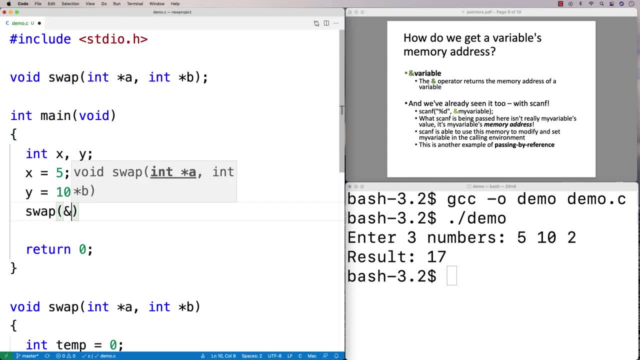 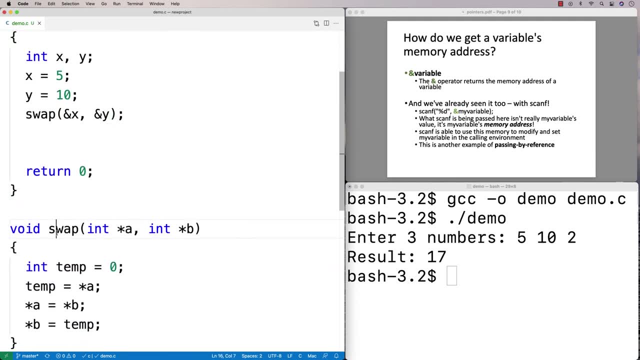 equal to 10, then i'm going to say swap and i'm going to give it and x and and y. now what's going on here is that we're not passing into swap the value of x and y, we're not passing in 5 and 10.. 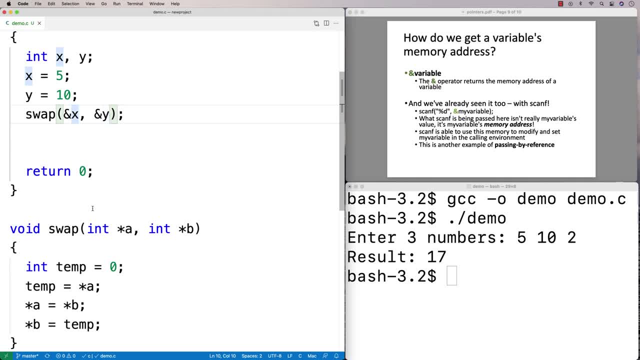 we're passing in the memory address for x and the memory address for y and swap is going to accept those, the memory address and the memory address. and a is going to be set to the memory address of x, b is going to be set to the memory address of y. then when i say, temp is equal to star a. 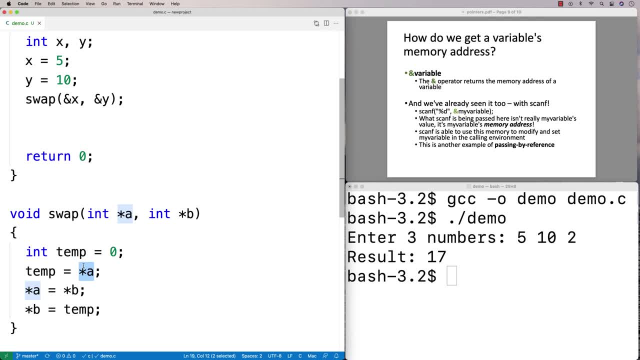 what's going on here is we're dereferencing the pointer and we're actually accessing, at that point, the variable x. because we're dereferencing the pointer, we're going to be accessing the variable x in the main function and we're going to be setting temp to that value there, to the value of that variable. 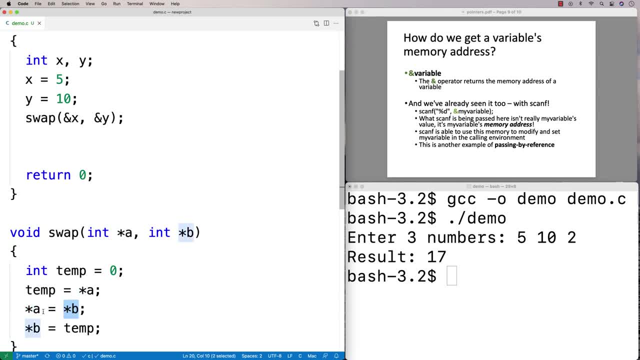 then we say star a is equal to star b. we're saying: go access what a is pointed to, set it equal to what b is pointing to. and we're accessing at that point the values contained inside x, y and we're setting them with the assignment here and we're using the 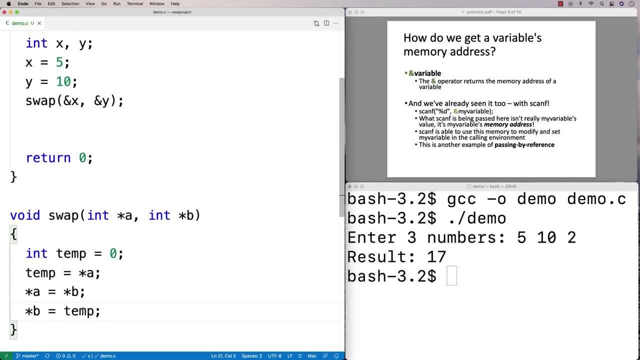 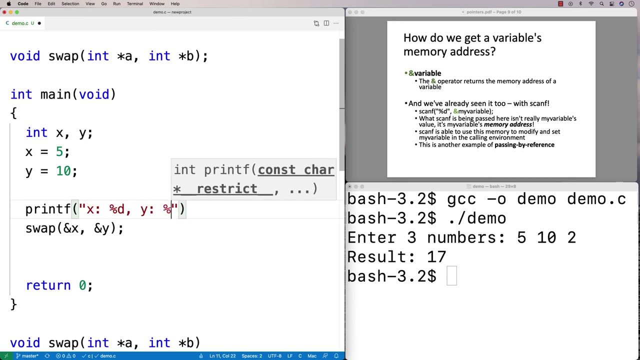 whacks. the one data arguments list and then we'll write somebody is the printf, and that's the node to printf that we have when we agree to the expression, then y is equal to tet'd and then all we do is consider our SGN characters. so we just block the stoic type statement from the. 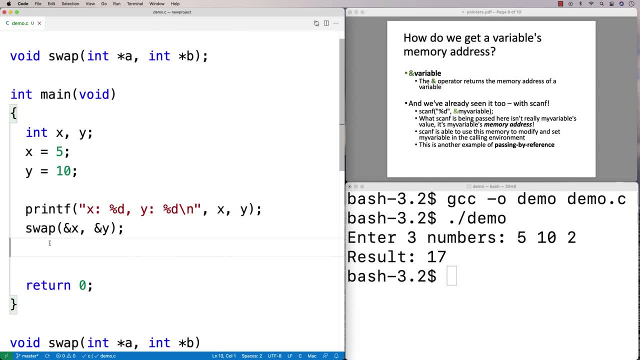 save and go close to thechiocom and then explicit this empty inhhhh one as limited to the lumped spec rédu зайло. in here we're able to just view: thisuito was finally when we say star b, x and y afterwards, and we'll just print this out and we'll just run this code here after we compile. 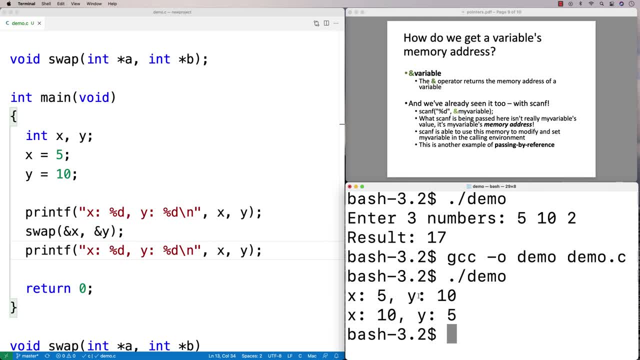 it and we get that x is 5 and y is 10. before and then after x is 10 and y is 5, and again, what's going on here that's key to understand is that we're passing in the memory address and that's. 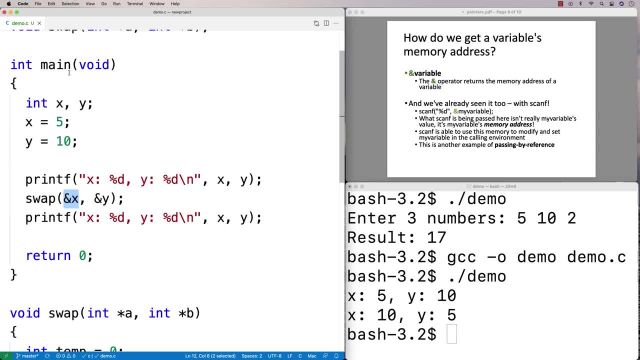 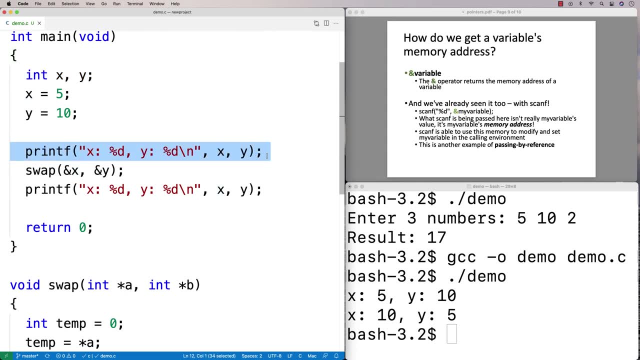 what allows swap to access both of these variables here in the calling environment main. so let's just do a printf actually of and x, and and y. let's do a printf of those values too. i'm going to print f and x and and y, the memory address of each. so i'll say percent p, percent p, and we'll print out and x. 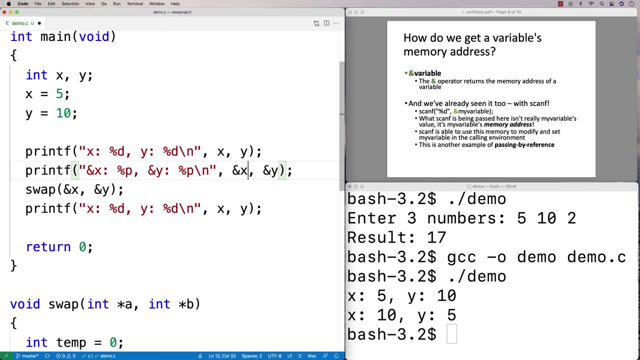 and and y, and what we're going to find- and i might actually put a new line between these as well, put a new line there, too- instead, what we're going to find is that they're going to be equal to a certain memory address that looks like the memory address that we had before for a and b, but what i'm also 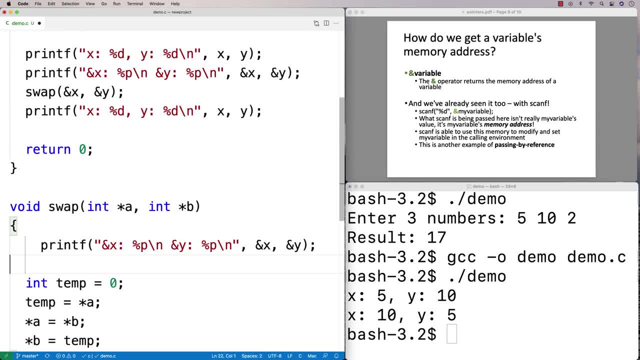 going to do is, inside this function here, i'm going to print f, the memory address of a and b, just that way it's it's clear what's being given to this function here. so i'm going to print out a and b, because a and b are. 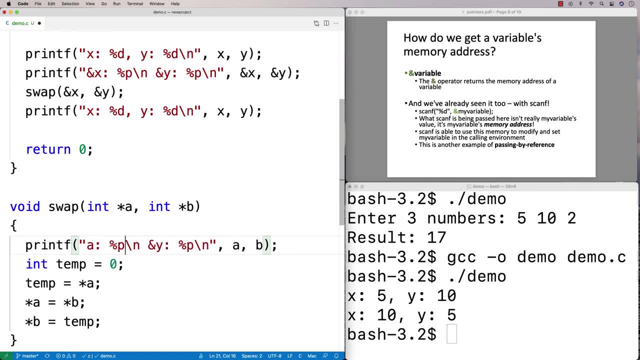 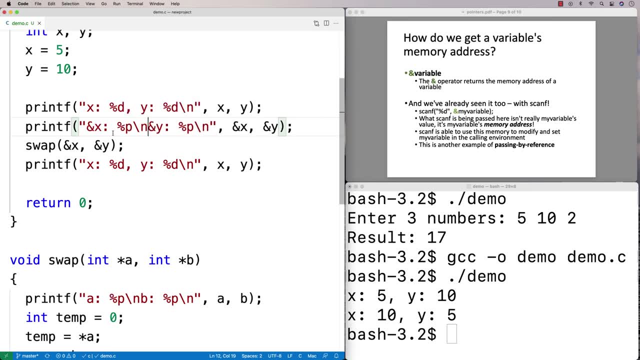 pointers that store a memory address. so i'll print out a and i'll print out b, and we're going to find that when we do this that a is set to the value of the memory address of x and b is set to the value of the memory address of y. so we'll say: gcc, dash out, demo, demo, dot c, run this. 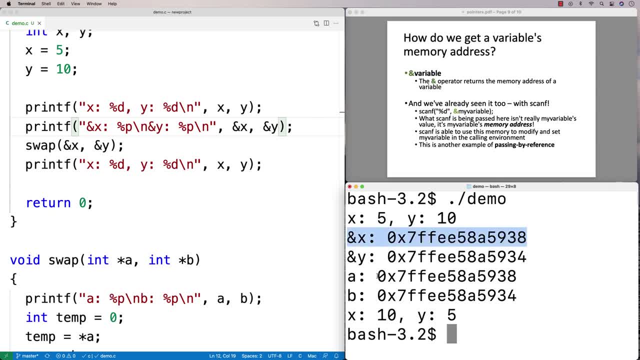 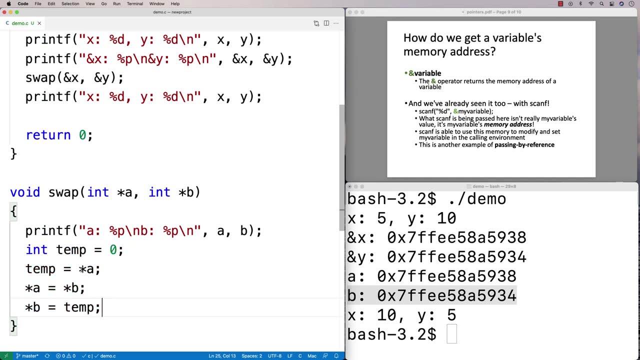 here and we get that, and x is this and a is this, and they're the same, and y is this and b is this, and they're the same, right, so? so what we did was we gave it the memory address of of those two variables there, and then what's happening in this swap is, when we say star a and star b, we're getting at the. 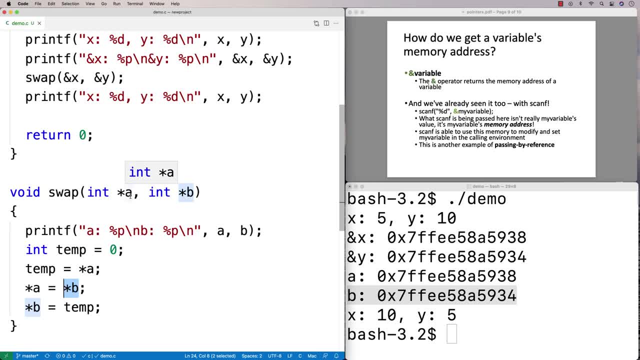 values that are pointed to by the memory address contained in a and b. we're accessing those values. so if i were to print f here, let's do a printf here of star a and star b. we'll say here star a, percent d, and we'll say star b, and we'll say percent d and we'll output. 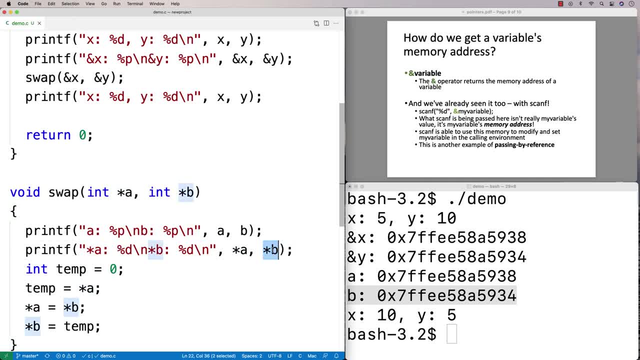 the, the value, what we get when we dereference the pointer a and dereference the, dereference the pointer b, and we're going to get what a and b are pointing to at that point. so i'll run this again and we get that a is 5 and b is 10 and it's not. it's not a, i should say. i guess i should say 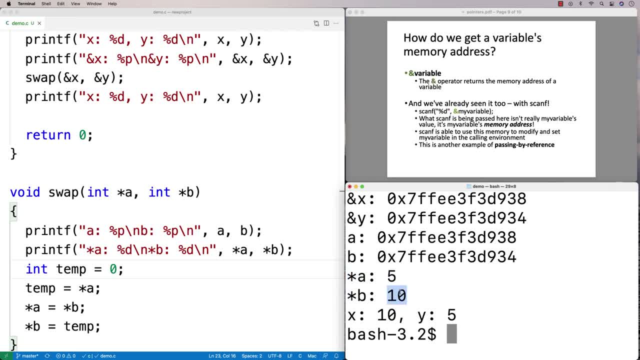 that it's. we reference a and we get 5. we dereference b, we get 10. right, and that's because when we dereference it, we go get what is at this memory address and x is at that memory address, and that's when we actually 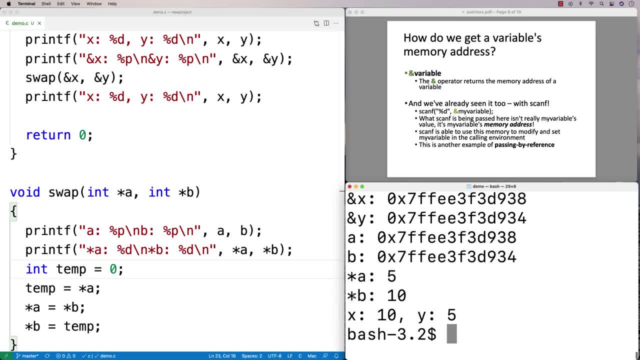 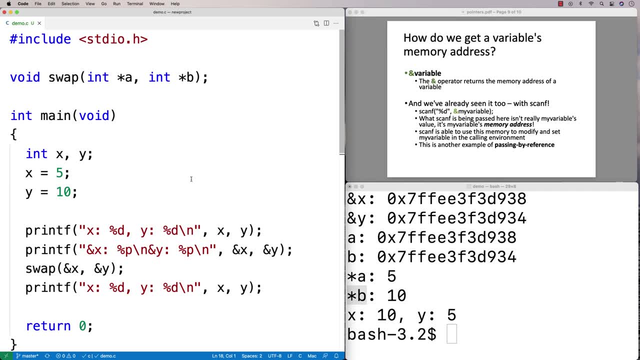 access the x value, we can access the y value similarly when we dereference b, and so that's what's going on there, and that's one of the things that a pointer allows us to do is to do this sort of pass by reference technique where we can have a function that is able to access and modify. 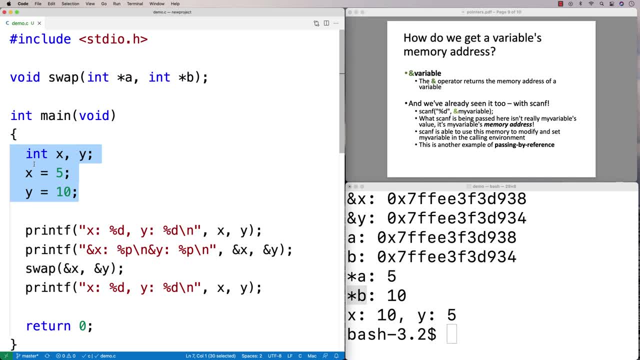 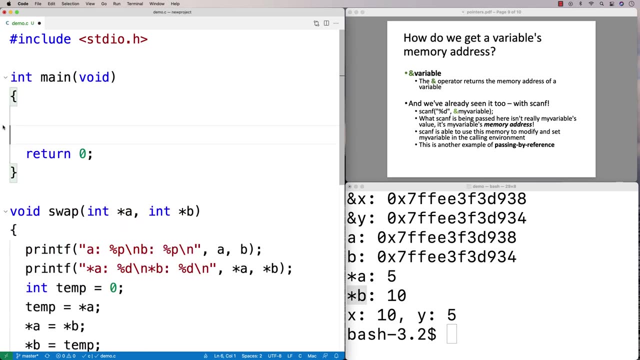 multiple variables in our calling environment for that function and alter them as it pleases, and that's again pass by reference, or more technically called pass by pointer. now the other thing that pointers allow us to do is what's called dynamic memory allocation, and dynamic memory allocation is where we want to have some chunk of memory that's allocated. 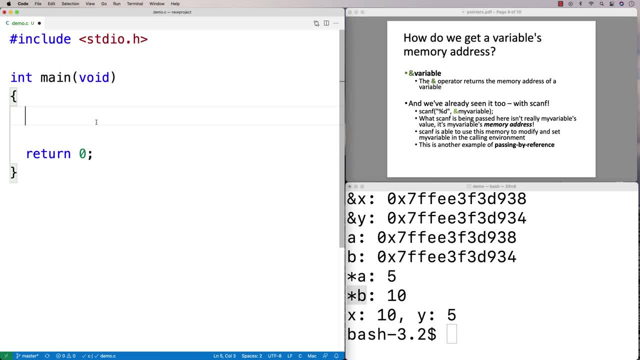 at at run time. so as our program is running, we decide to allocate a certain amount of space at run time. so if i normally declare an array, say in c, i could say like int a is 10 and at at compile time. here what's happening is i'm deciding to have an array that is going to be of length 10.. but what if i 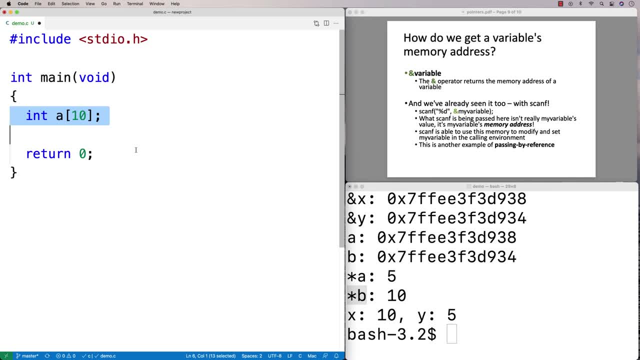 don't know at compile time, when we compile our program, how large of an array i need. what if i ask the user like, hey, how many employee salaries do you want to enter? or you know how much of this kind of data do you need to require? you know how much of this kind of data do you need to require? 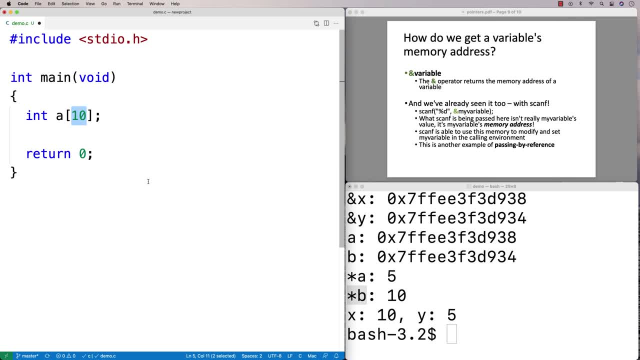 to record. at that point i might need to allocate space dynamically at run time, as my program is running, and that's where dynamic memory allocation comes in. and again, i'm going to make another tutorial video on this because it's a big enough subject, but i wanted to put in this pointer video. 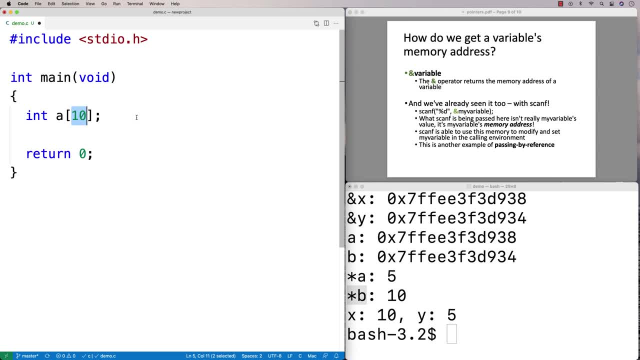 too, just to give you another example as to why pointers are useful. so what i can do is this: i can say here: hint star a, and this is going to be a pointer to what we're going to call a dynamically allocated array, and what I'll do is I'll have a size of that array, so I'll say like: 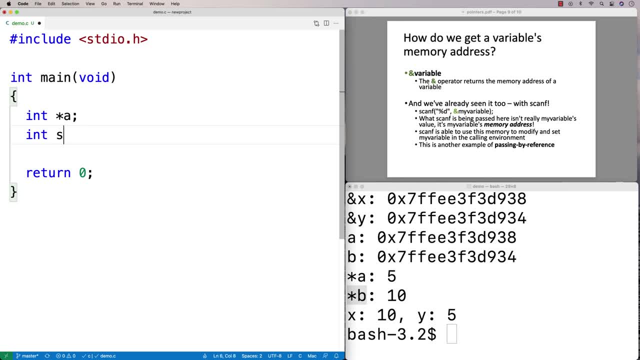 int size, maybe I'll call it length. I'll say int length, I can initialize it to zero and I'm going to ask the user to enter a length. so I'll say like printf. I'll say enter a length and then we'll do scanf and we're going to store the length. we'll say percent d and we're going to store the length. 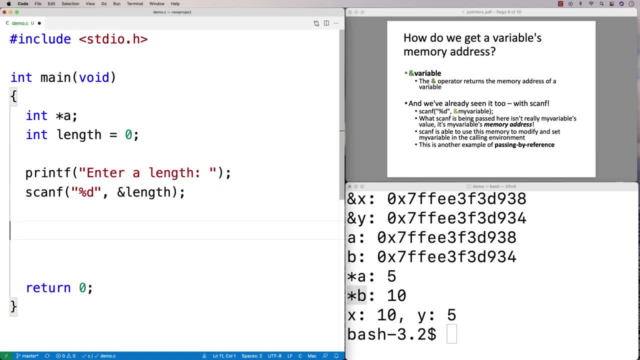 that they enter into length. what I'm going to do is I'm now going to allocate space dynamically for an array of this length. so what I'm going to do is I'm going to say a is equal to, I'm going to say malloc and I'm going to say length times size of int. now, what's going on here is malloc. 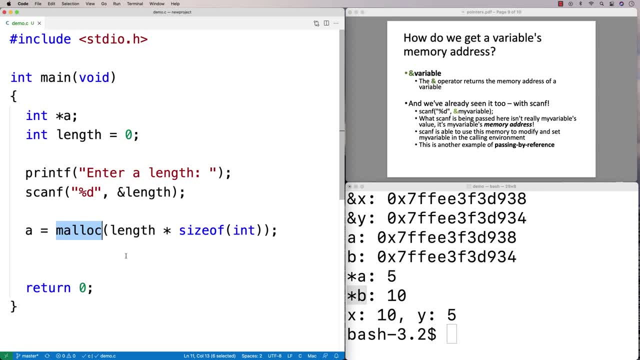 is a function that actually allocates space on what's called the heap. the heap is the area of memory that's for dynamically allocated things and it's actually, if we think of our visualization here, it's actually kind of located at the bottom here. this here is what's called the stack, and it goes downwards. the heap is actually kind of at. 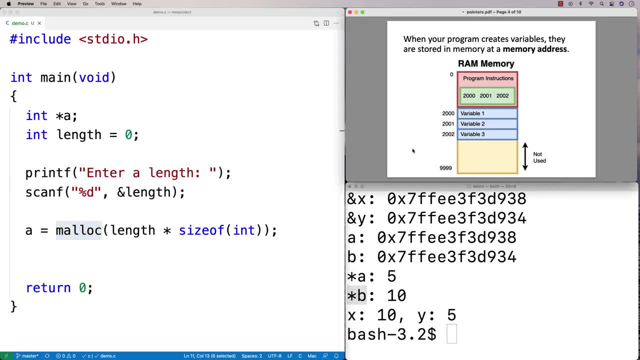 the bottom here and it grows upwards. we can think of it like that, anyways, and what we're going to do here is we're going to actually have a be a pointer to that newly allocated space that's been set aside for us, and what malloc takes in as an argument is how much space. 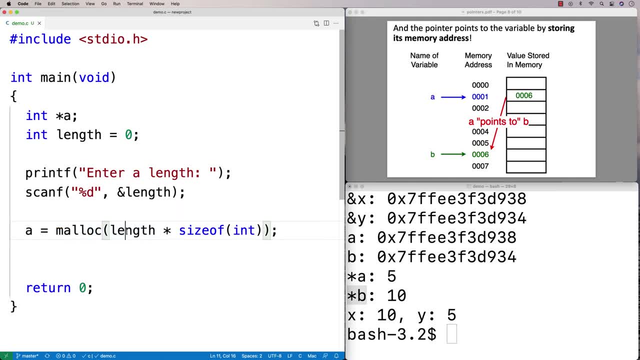 do you need in bytes? how many bytes do you need? and we're saying we need the length, so we need this amount of space times the size that it takes to store an integer, and malloc is then going to give us that memory that we can then work with to do things like store data inside of it. so I 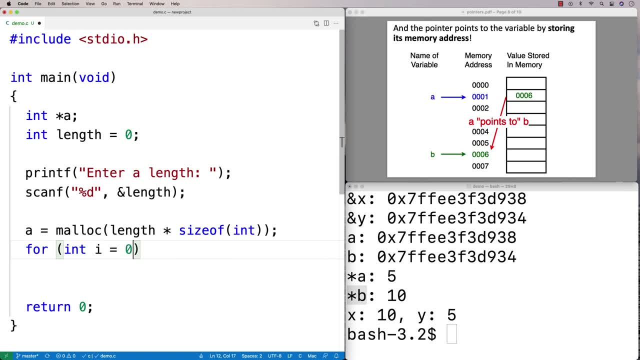 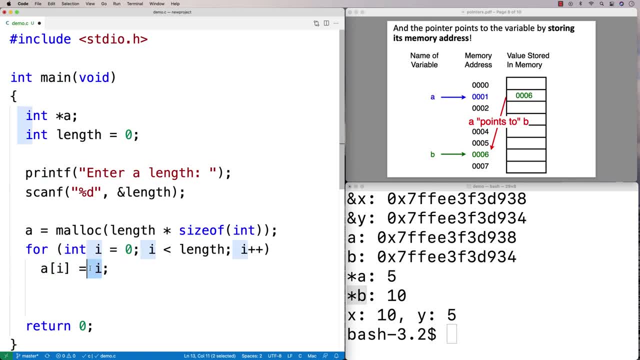 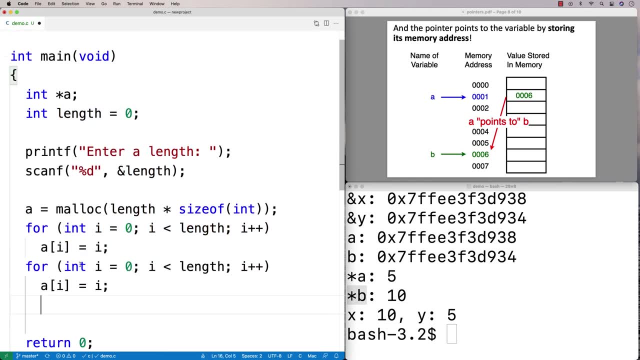 going to store in a at position i the value i. so we're going to store from like zero up until the length that we've decided here, and I could print it out too. so I could like store some values in there and I could print it, print out things as well. so I'll say: store some values and I'll do. 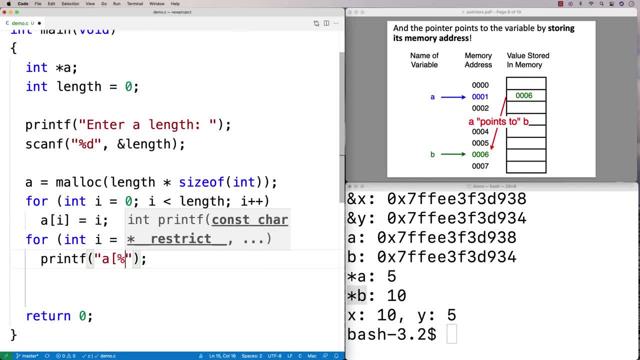 some printing years too. so I'll say print f and I'll say a percent d is equal to percent d and I'm going to output the values that I just stored. so this will store some data for us in that newly allocated space. this will print out the values in that newly allocated space and when you're done working with data, 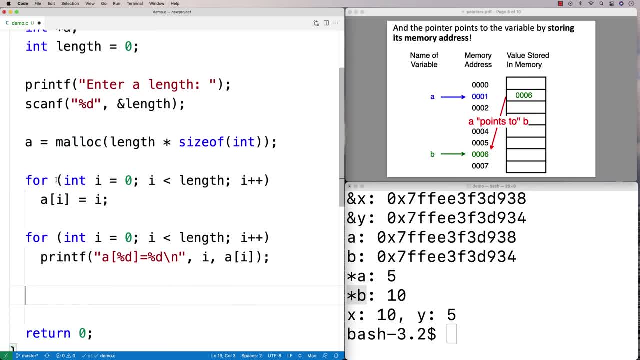 that's been dynamically allocated, you have to free the space, the allocated. so I'm going to say free a and what this does is it makes that dynamically allocated space available again. if it were to be, if it needs to be allocated again, say it's now free to be allocated again if I, if I don't free. 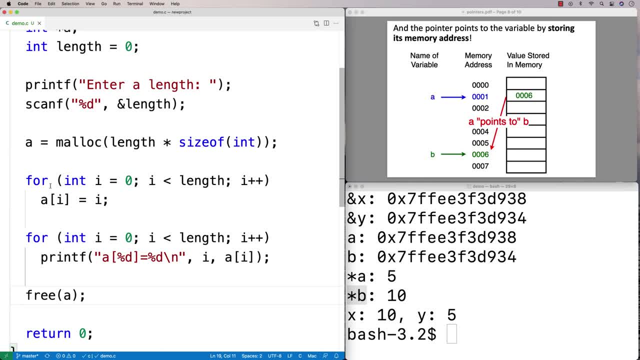 it. I have what's called a memory leak, where I've got some memory that you know can't really be used at that point, and so we have to free the space after you've allocated it. but in this case a a is again going to be a pointer. so if I were to do a print- print f here, and I would say: 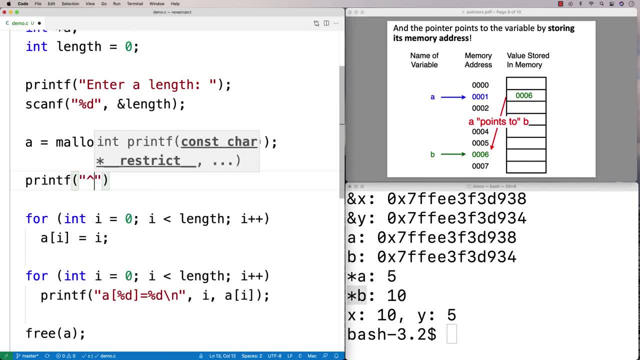 like print f and let's say: let's print out and a. I'll say: or actually I'm just going to print out a, I don't need to print out and a because a is a pointer. I'll say: print out a percent p and we'll. 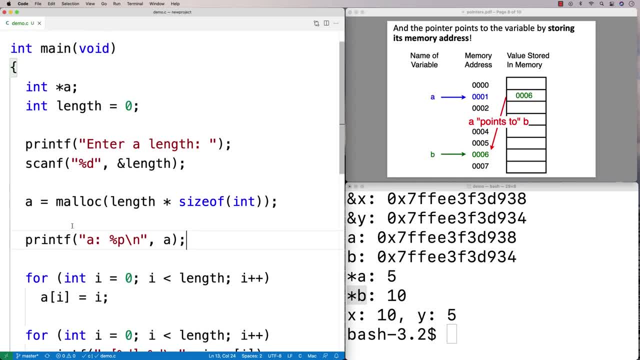 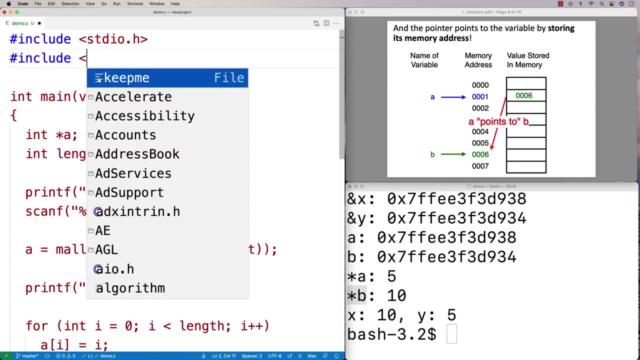 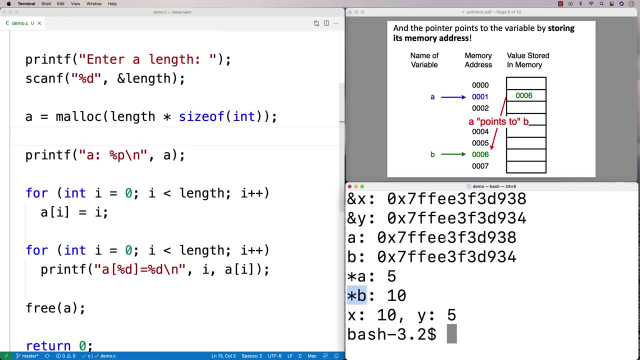 print out a there. okay so. and the other thing I have to do is because I'm using malloc, I have to include one more library. I have to include std libh, so number include std libh, because I'm I'm going to make a memory address so I can inside my library. I'm just going to call malloc. 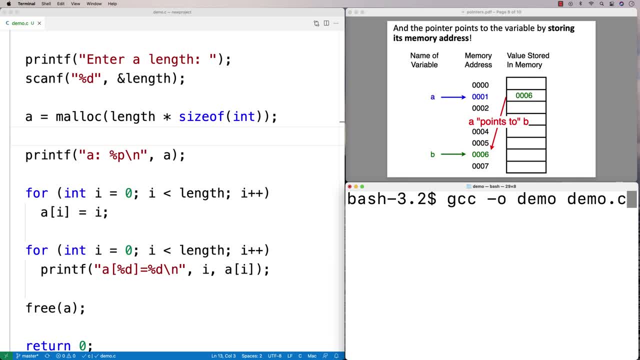 where I'm going to click, so and I'm going to call them and I'm going to say they're just going to come up and hover this way. so in this case it's a abt this way that I'm saying that I'm going to call the library. that's where I want to store this memory, to store this memory. 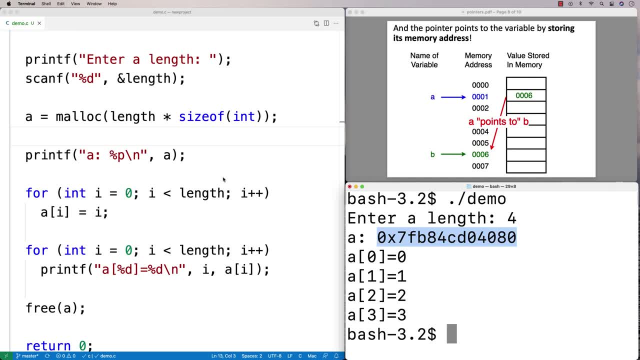 and if I do that I will be able to actually save. so I go back to my library and I go into there and I go to- if I just wanted to show a memory address in here, and I go ahead and select that and then pretty much I'm going to just save. so I'm going to just go ahead and just